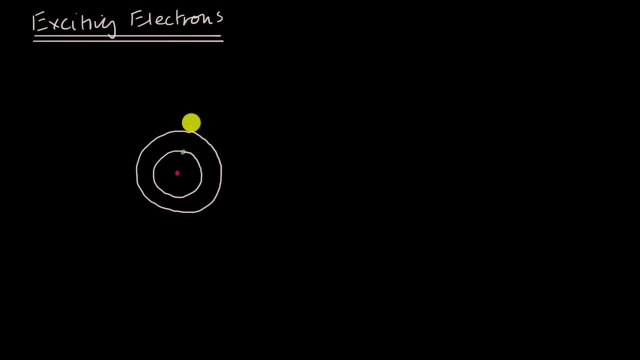 but it can be excited to other shells. It could be excited to the second shell or the third shell or the fourth shell, and this is obviously hand-drawn and not hand-drawn that well, and this is really just to help us. 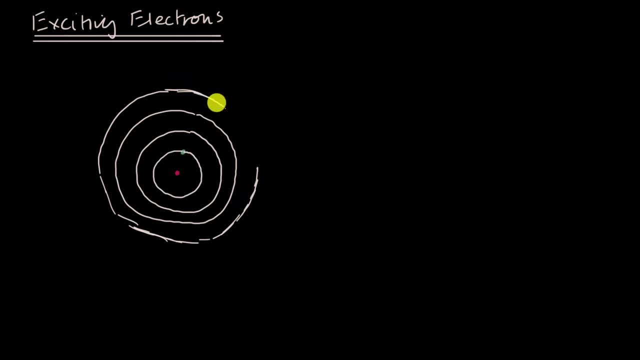 for visualization purposes. We know that electrons. electrons don't orbit nuclei the way planets orbit stars. They're really more. they have both particle and wave-like properties and they're more of a probability density function of where you might find them. and these energy levels are associated. 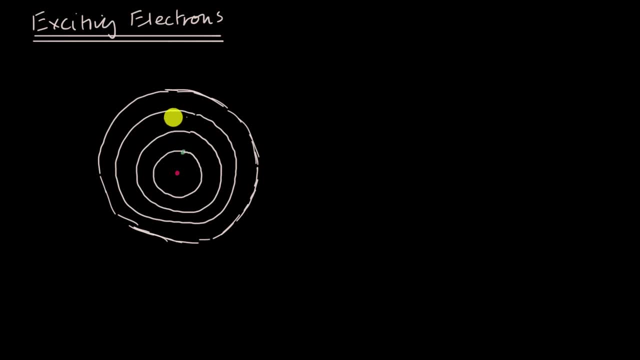 with different probability densities of various energies. but this is what an electron will typically look like if we're thinking about just a neutral hydrogen atom, where the electron's in its ground state. Now, let's say we're dealing with a hydrogen atom where the electron has already been excited a little bit. 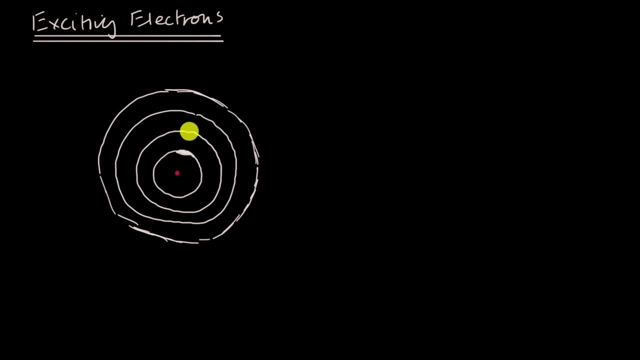 so, instead of it being in the first shell, it's already in the second shell, right over here, and what we're going to do is we're gonna hit it with a photon that excites it even more, and the photon- and we know that light. 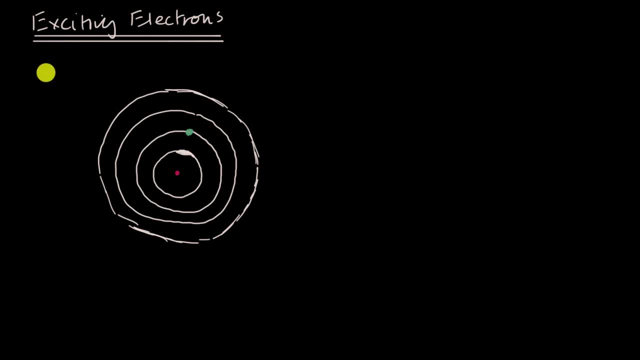 has both particle and wave-like properties. When we think of it as a particle, we think of it as a photon, but I will depict it like this. so this light has a wavelength of 486 nanometers, and we know that that wavelength 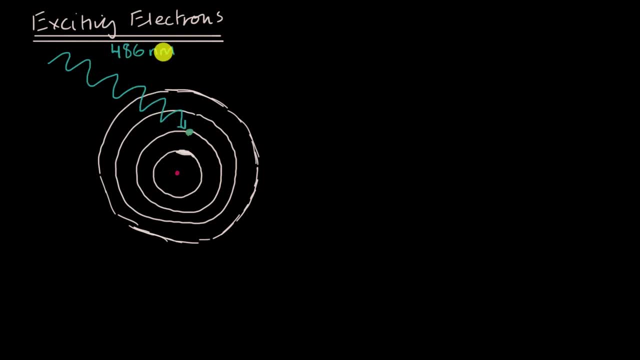 that photon that hits it with a wavelength of 486 nanometers has sufficient energy to excite this electron, in this case actually, from n equals two, from the second shell to the fourth shell, so it'll go all the way over over there. 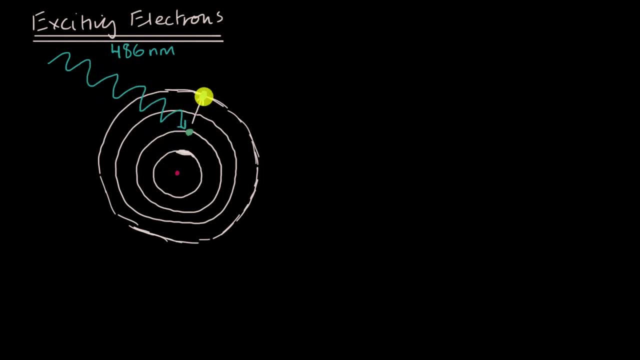 so it will absorb that photon and then after some time it can come back down. and when it comes back down I could do it over here. so after some time it can that electron right over here, that excited electron, it can go back from the fourth shell. 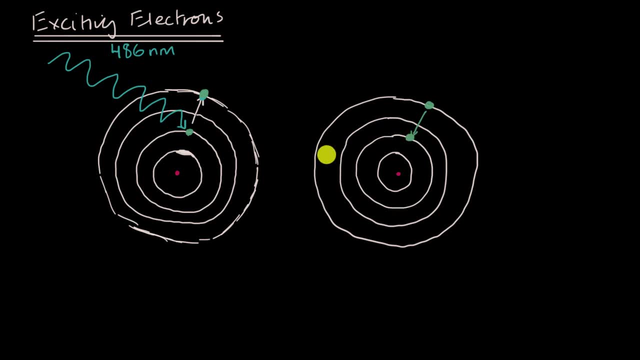 to the second shell and when it does it, it will emit a photon of that same wavelength. so as that does that, it will. it will emit a photon of 486 nanometers. so, just like that, we already are starting to understand. 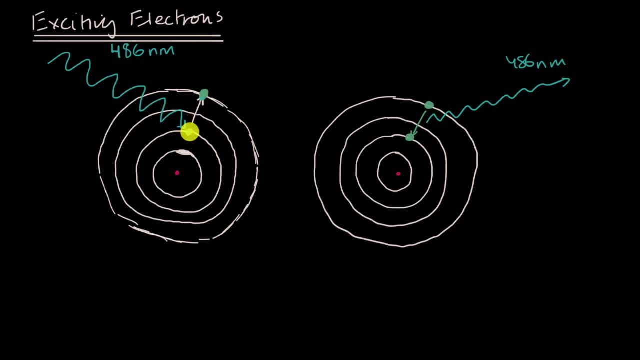 that photons of the right energy can excite an electron, and that's the same thing we're talking about when we talk about quantum mechanics. is this notion that photons need a certain amount of energy in order to be able to excite the electron to the next energy level or the energy level after that? 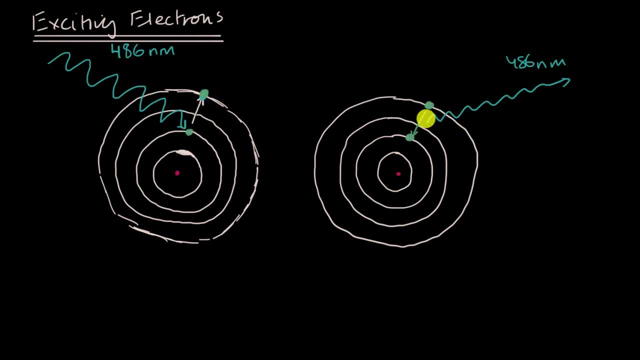 Things in between don't work, and the same thing is true when you're emitting the energy. The electron's not gonna go from the fourth energy level to someplace in between the fourth and the third. It can't do that. It has these quantum states. 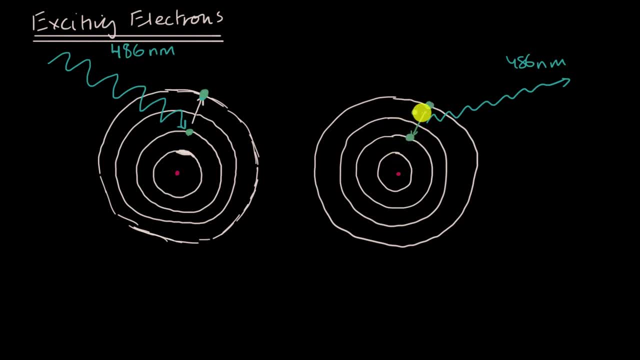 It's going to be there in the fourth or the third or the second or the first, not at the. there's no such thing as a 3 1⁄2 shell and we can actually answer based on this. 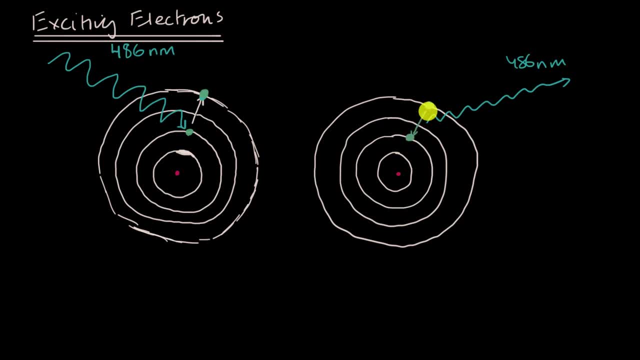 We can think about what is the energy difference between these shells? and the energy difference between these shells is essentially the energy of the photon that we emit when we go from the fourth energy shell, from the fourth shell, to the second shell. To figure out the energy of that photon, 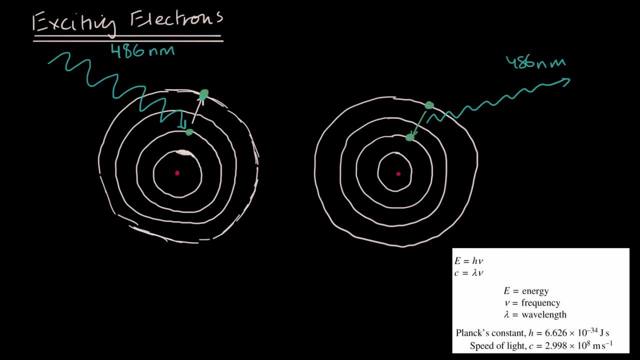 we just have to think about some useful formulas in quantum mechanics. The first, and I'm gonna just look at it right over here- is that the energy is equal to Planck's constant times, the frequency. So this thing that looks like a V. 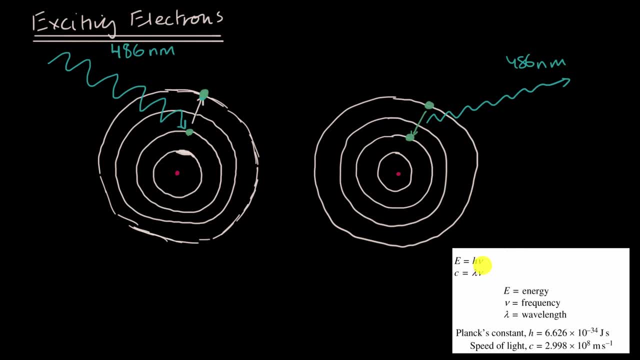 this is actually the Greek letter, the lowercase Greek letter, nu, and this is what we typically use for frequency, especially when we're talking about frequencies of things like light. and we also know how to go between frequency and wavelength, because we see that the speed of light 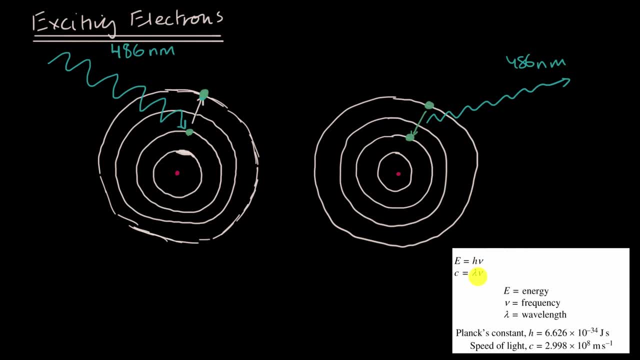 is equal to whatever the wavelength of that light is, times the frequency of that light. So how would we figure out the energy of one photon, a 486 nanometer light? Well, we could think about it this way: We can first figure out its frequency. 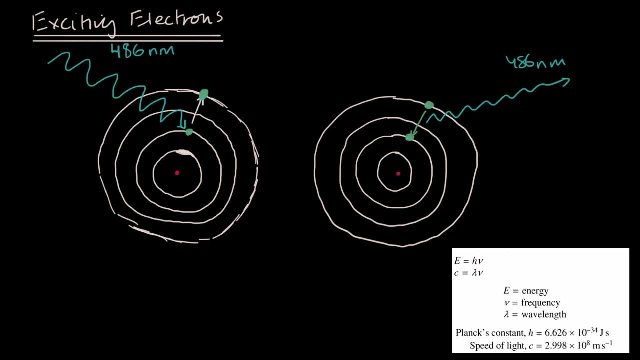 using C is equal to lambda times. nu Let me write this down. So we know that C- the speed of light, is equal to the wavelength of the light times the frequency of that light. And so if we know the wavelength we can figure out the frequency. 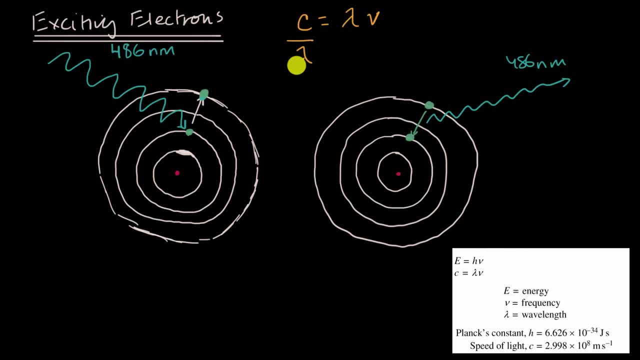 by dividing both sides by lambda. So let's do that. So if we divide both sides by lambda, we get that the frequency of the light is going to be equal to the speed of light divided by the wavelength of the light. And remember, they've given us 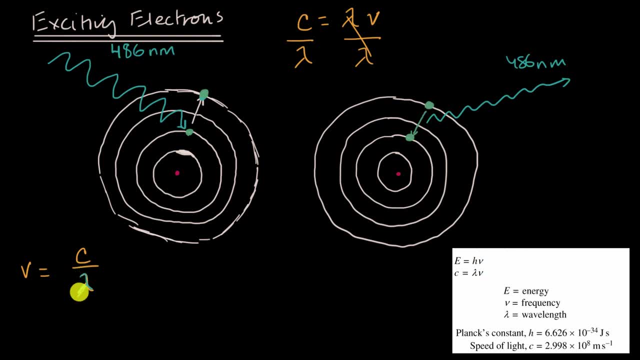 the wavelength of the light here 486 nanometers, or at least I have given it to you. And then you could take this and plug it back into Planck's equation. up here that energy is equal to Planck's constant times, the frequency to figure out the energy. 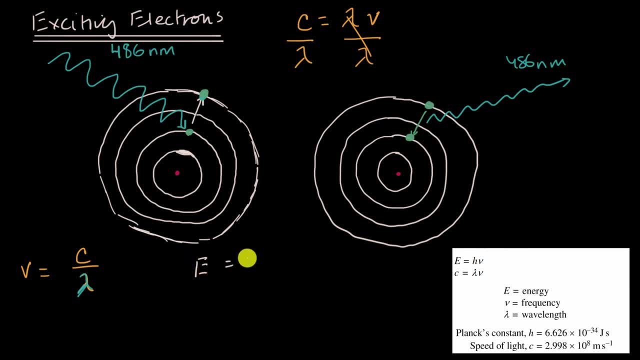 So let me write that down. So the energy is going to be equal to Planck's constant times. the frequency: Well, we know the frequency right over here. so it's going to be equal to Planck's constant times. the speed of light. 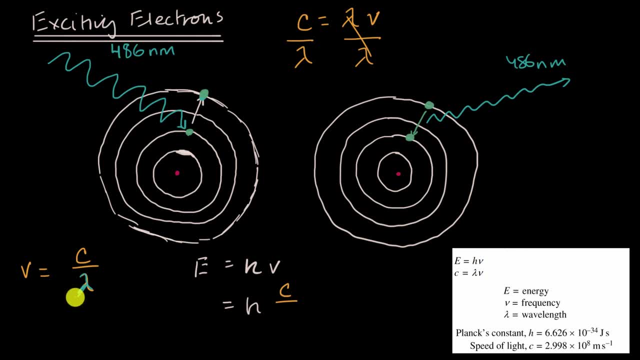 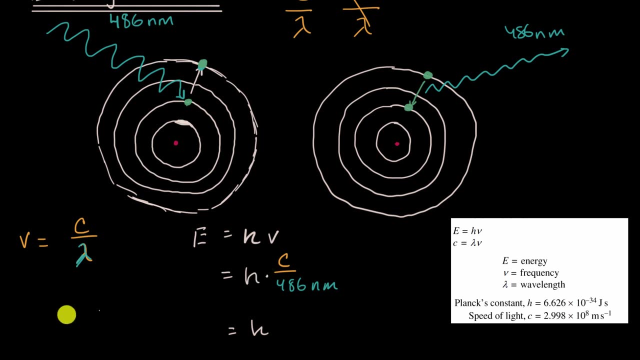 divided by the wavelength of our light, which we know is 486 nanometers. 486 nanometers, So we could say, just scroll down a little bit- that the energy is going to be equal to Planck's constant times. the speed of light divided by the wavelength. 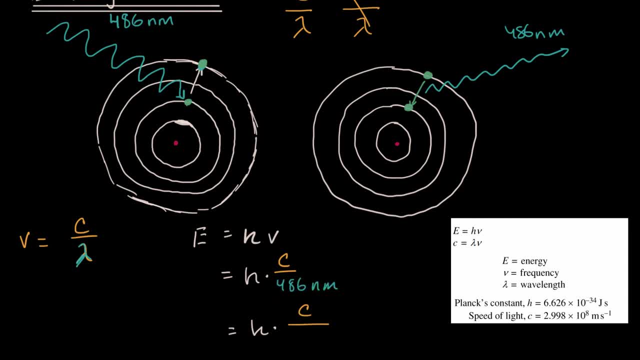 divided by. instead of writing the wavelength as 486 nanometers, I can write it as 486 times 10 to the negative ninth meters. A nanometer is just one billionth of a meter, And then we can just get our calculator out. 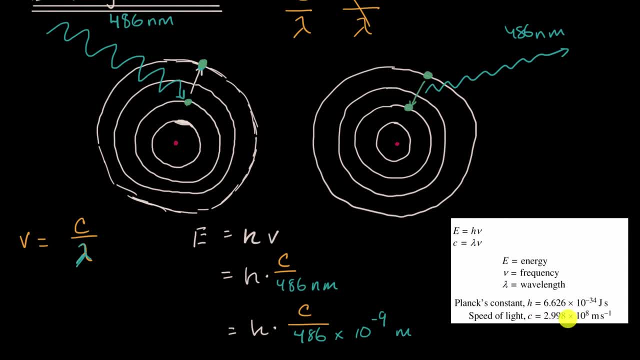 and we know what Planck's constant is. They give it right over here. We know what the speed of light is right over here And we know that we have a maximum over here. They're giving us four significant figures in each of these. 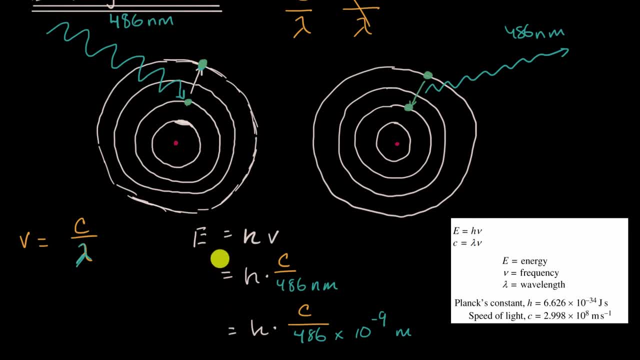 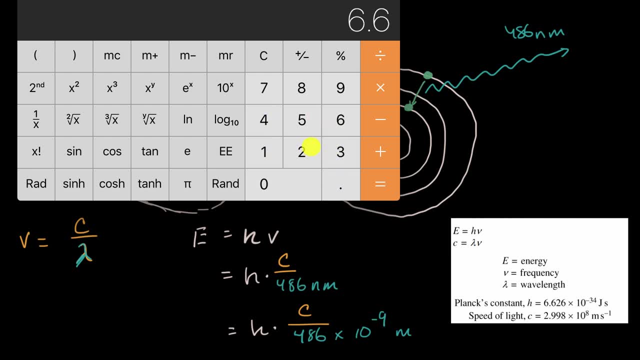 And then we have three significant figures here. So our answer is going to be in terms of three significant figures. I'm going to get Planck's constant, which is 6.626 times 10, to the negative 34th joule seconds. 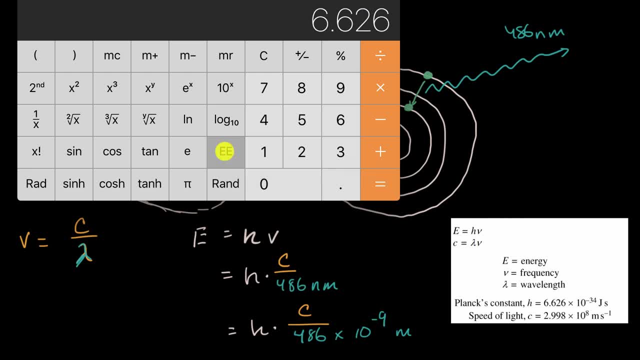 So let me write that down. So times 10 to the negative 34th, And I'm going to multiply that times the speed of light, So times 2.998 times 10 to the negative 34th. So times 2.998 times 10 to the eighth meters per second.